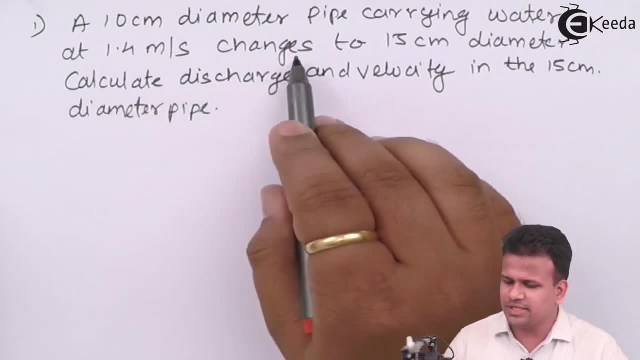 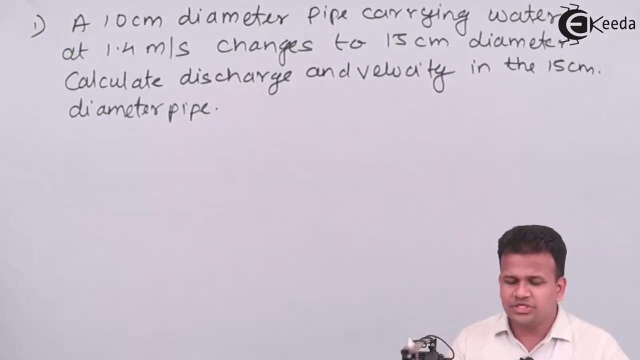 at 1.4 meters per second changes to 15 centimeter diameter. So there is a pipe in which the initial diameter is 10 centimeter and the final diameter is 15 centimeter. During the course of the length of that entire pipe the diameter is increasing. That means the area of cross section is increasing. 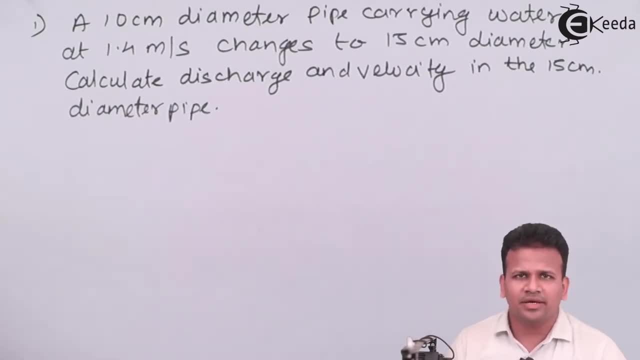 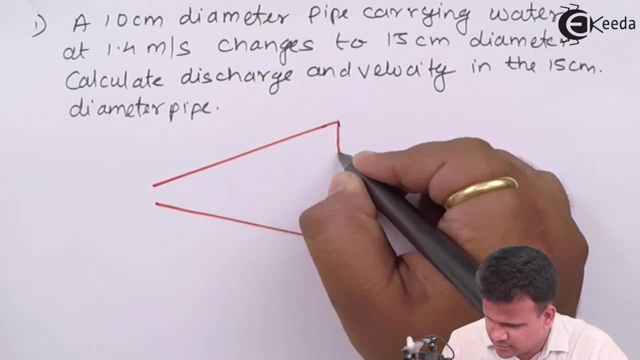 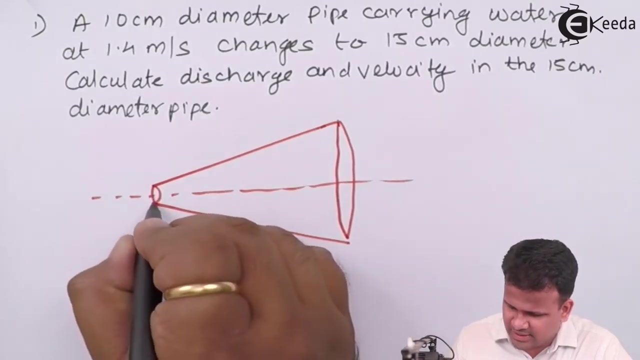 So let us draw a diagram for this entire problem. So there is a diameter of the pipe, So let us consider this as having a diameter. d1 is equals to 10 centimeters, So that can be written as 10 into 10, raised to minus 2 meters, So that is 0.1 meters. 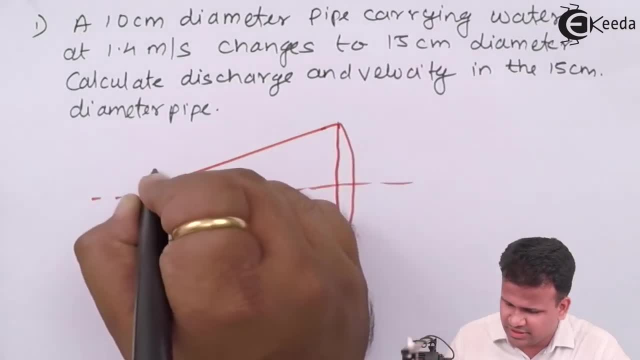 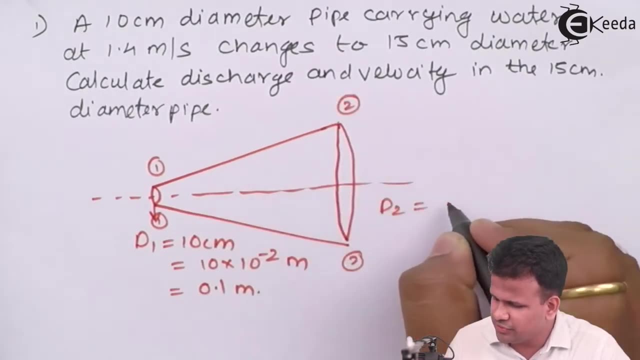 At this section. let us first consider this section as section 1.1 and this as d1 is equals to 1.2 meters. So let us consider this section as section 1.1. section 2: 2 at section 2: 2 diameter. d 2 is 15 centimeters, that is 15 into 10 raised to minus. 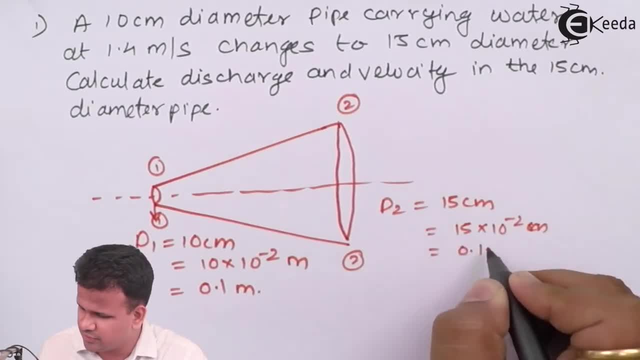 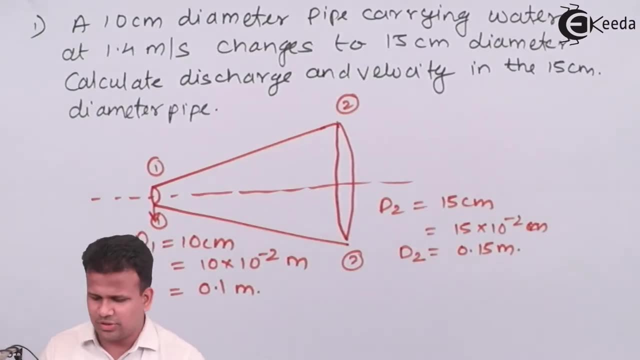 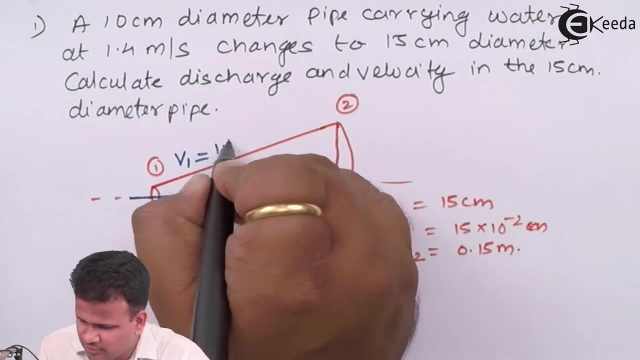 2 meters, that is equals to 0.15 meters, that is section diameter at section 2.. Now, during the course of this, the fluid is flowing from section 1: 1 at a velocity v 1, which is equals to 1.4. 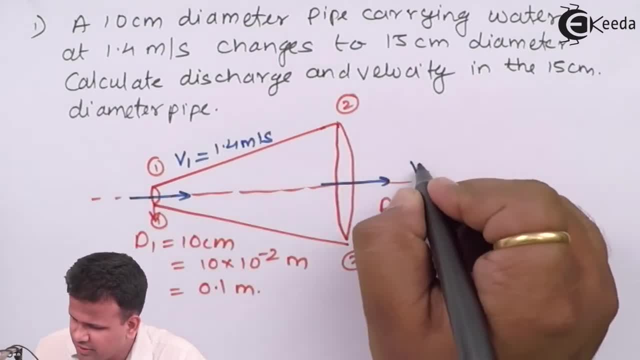 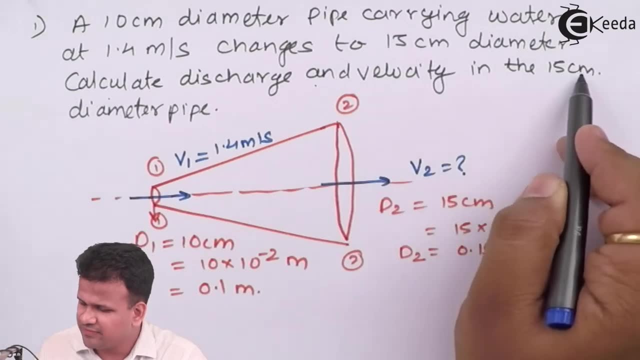 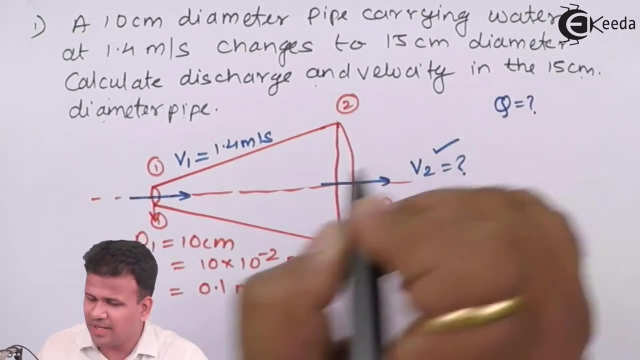 meters per second and the velocity v 2 is unknown over here. What they have told you to calculate, calculate the discharge and velocity at 15 centimeter diameter pipe. So we have to calculate the velocity v 2 as well as the discharge in the pipe. So now let us calculate this. So, according 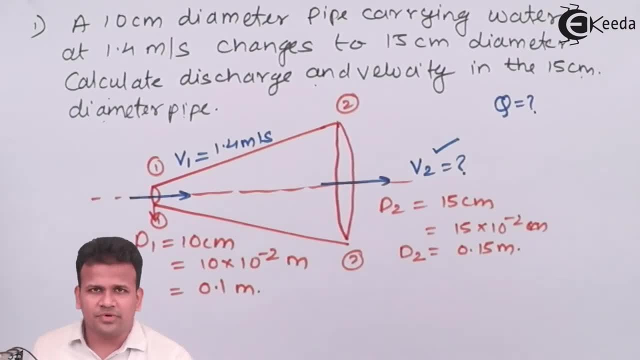 to the continuity equation for an incompressible fluid flow. we know that a 1 v 1 is equal to equals to A2- V2.. Now, out of all these terms, what we know over here is term V1.. We don't know term. 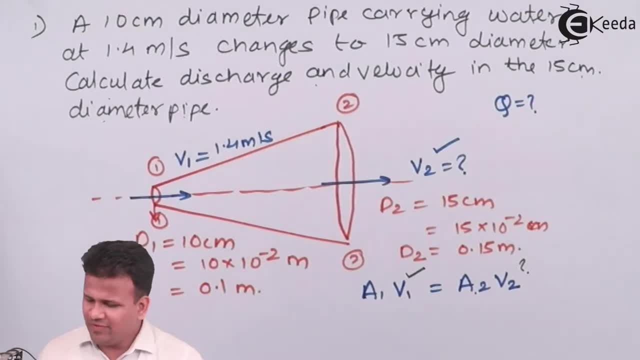 V2.. A1 and A2 is also unknown. A1 and A2 can be calculated by this. A1 and A2 can be calculated with the help of diameter D1 and D2.. So let us calculate the value of A1 and A2.. 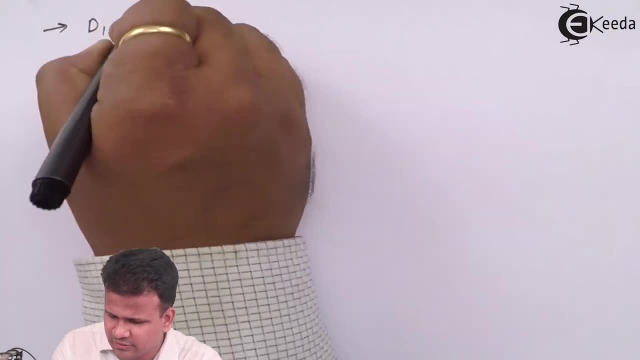 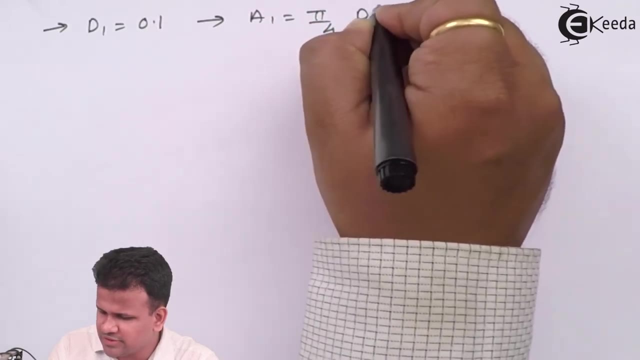 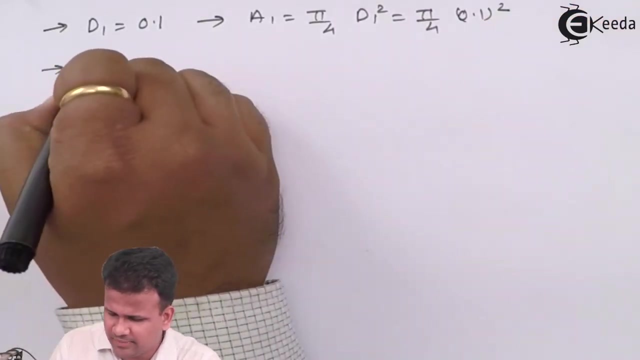 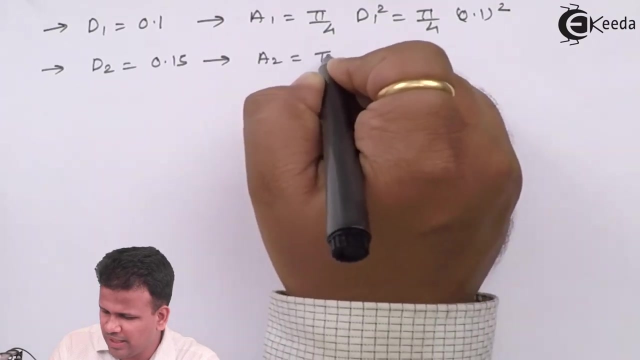 So for diameter D1 is equals to 0.1, area A1 will be equals to pi by 4 into D1 square, that is, pi by 4 into 0.1 square, and diameter D2 is equals to 0.15. area A2 is equals to pi by 4 into D2 square. 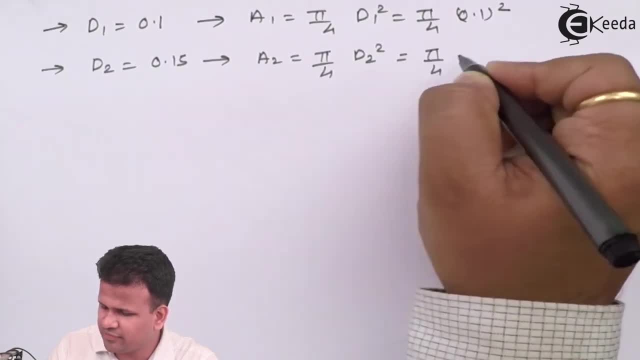 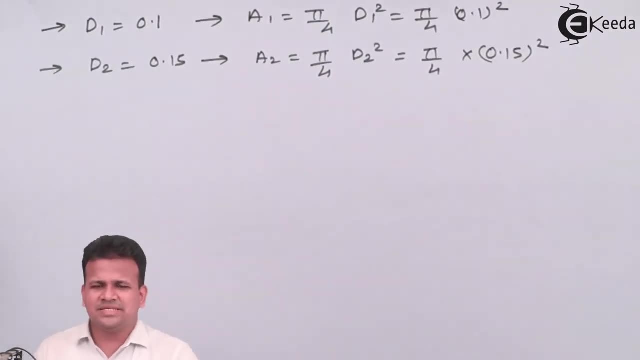 that will be equals to 0.1 square. So for diameter D1 is equals to 0.1 square, area A2 is equals to pi by 4 into 0.15 square. Now, without calculating this, let us directly substitute that in a: 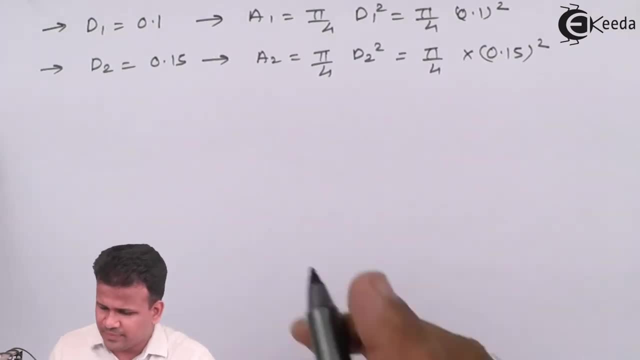 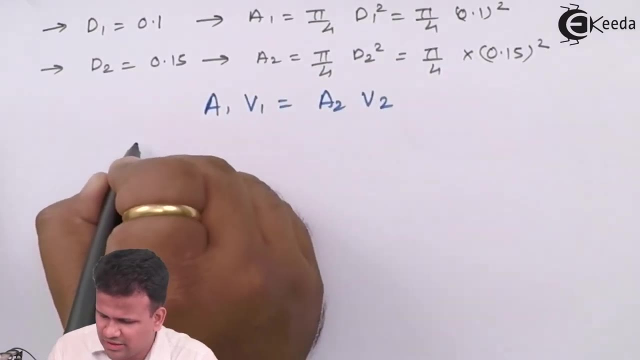 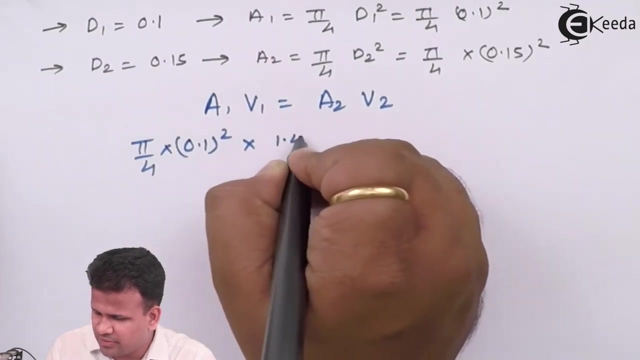 continuity equation. So what do we get this? as that is first equation, A1- V1 is equals to A2- V2.. So A1 has a value of pi by 4 into 0.1 square. V1 has a value of, that is, 1.4.. A2 has a value of: 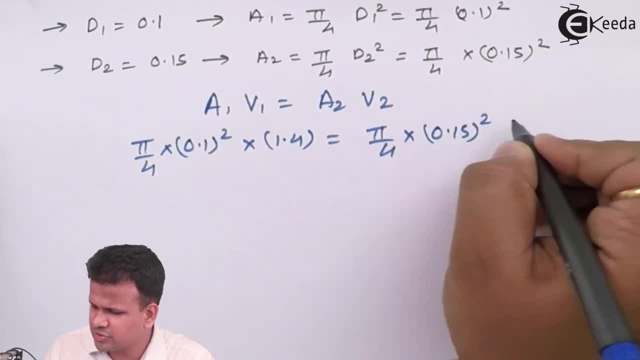 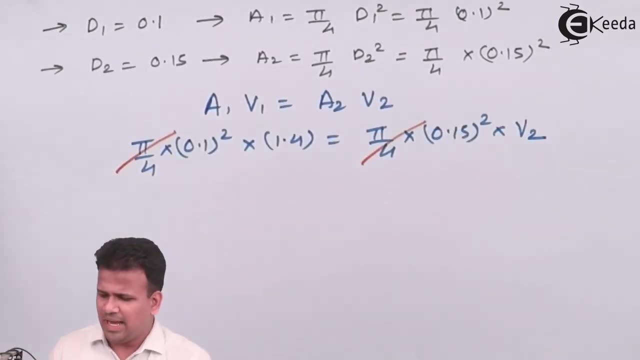 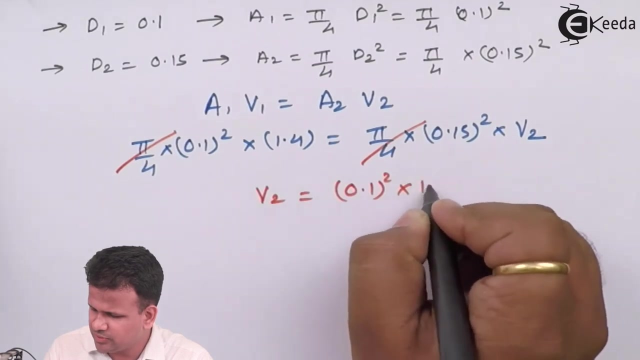 pi by 4 into 0.1, the whole square into V2.. Here the terms pi by 4 and pi by 4 can be cancelled and we will get: V2 is equals to 0.1, the whole square into 1.4 upon 0.15 square. 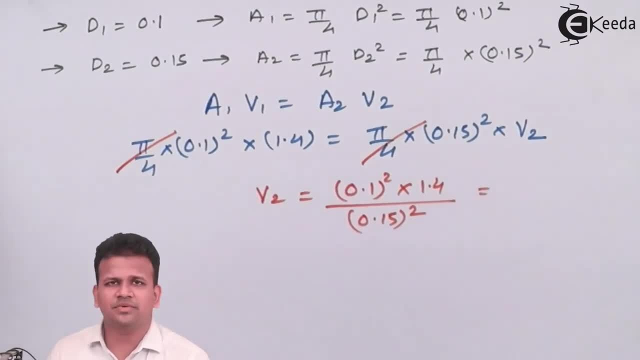 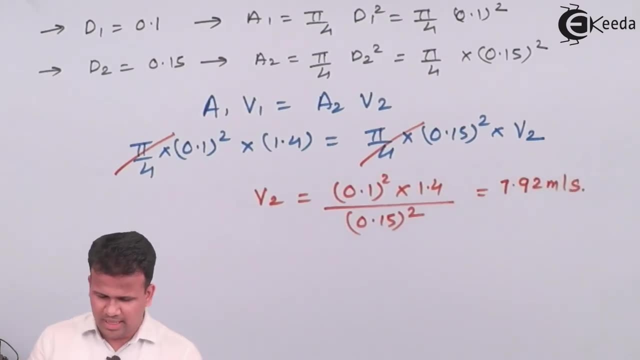 So here the value of V2 is equals to 7.9 per second. Now we have calculated the value of V2.. Let us calculate what is the discharge. So discharge can be written as A1- V1 is equal to A2- into V2.. So now let us calculate what is. 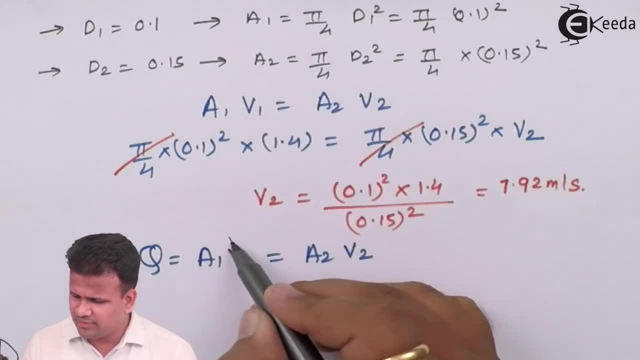 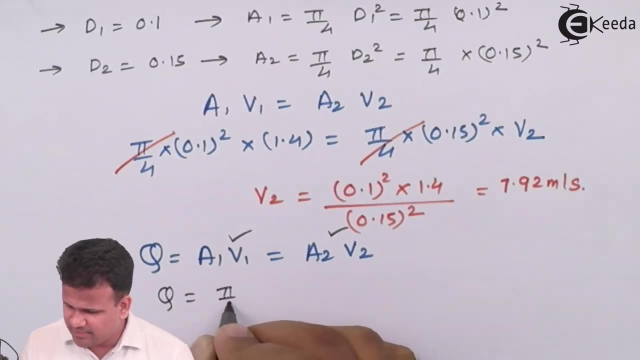 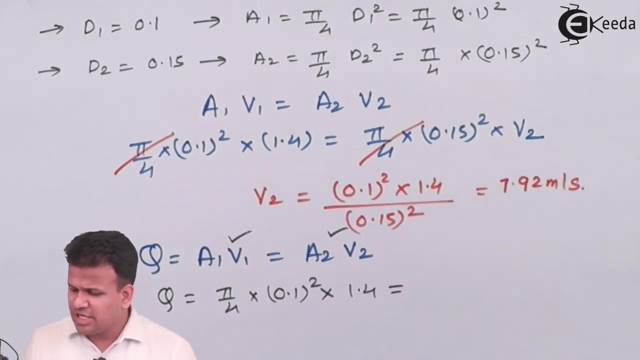 the discharge. You can calculate discharge either by A1 V1 or by A2 V2.. Let us take the first term, that is A1 V1. that is pi by 4 into 0.1, square into 1.4.. The value of discharge comes out to be: 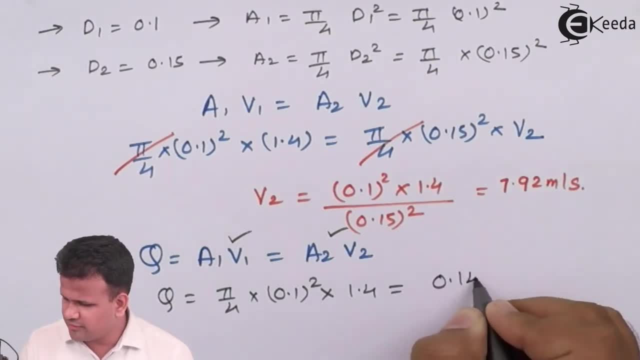 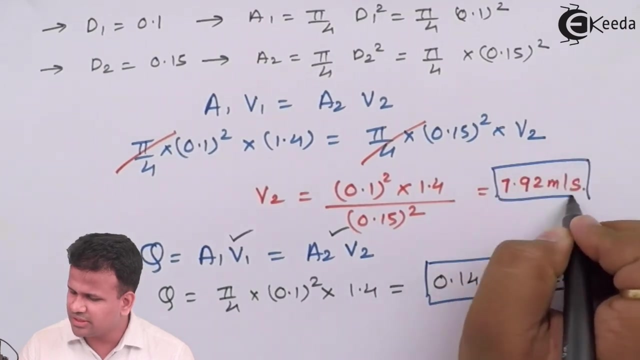 0.14 meter cube per second. So we have calculated the discharge- that is 0.14 meter cube per second. and as well as we have calculated the velocity at the outlet. That is 0.14 meter cube per second. So we have calculated the discharge. that is 0.14 meter cube. 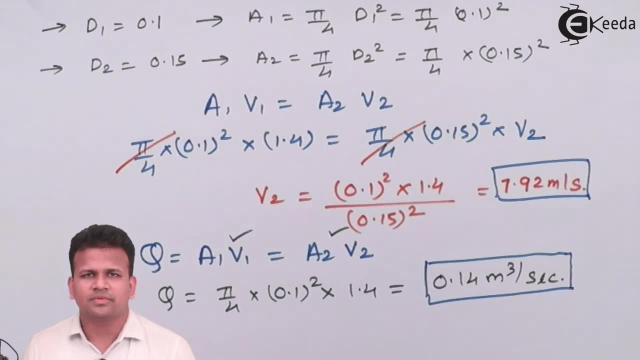 that is at section 2.2.. Thank you.